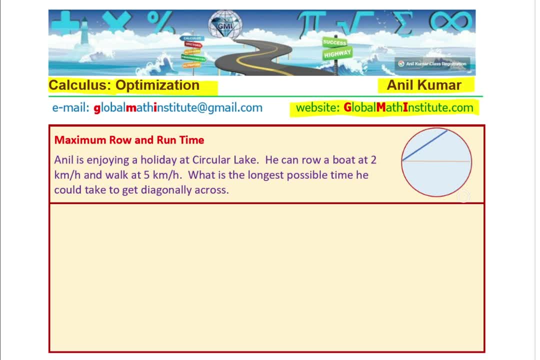 on the right. So that is the Circular Lake right, And let us see how it unfolds. And let us say Anil is in position A and wants to go across B. right, We are given the rowing and the running either walking speed of Anil, So one way, of course, that he can go straight. 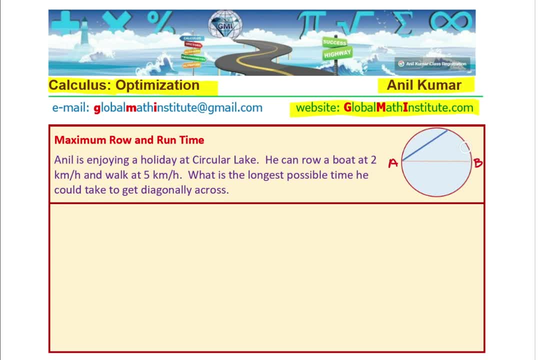 right, Or he could just walk along the lake. And third, he could actually go to some point, let us say C, and then walk along the beach. You see that That could be the third option. You can definitely find the times A to B and A to C and also from A to C to B right. 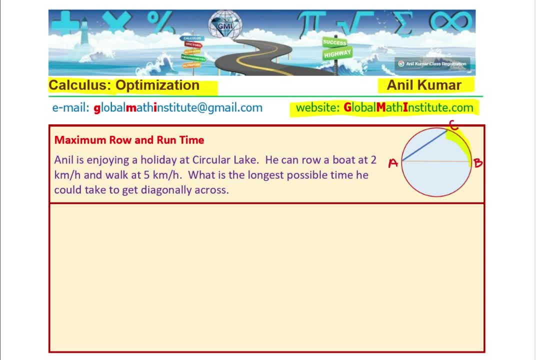 Now the thing is, how do we figure out which path to follow so that he gets maximum time enjoying in both rowing and walking right in this particular time before he reaches point B? That is the whole idea. Okay, If you have got the question, feel free to pause the video and answer it. 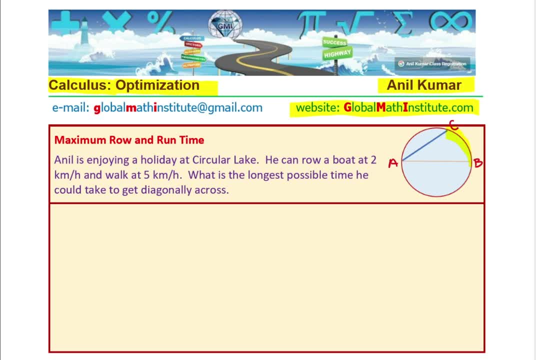 Perfect. So let us write down the information given to us and what is required and see how can we relate all these things right So we can say that the velocity for boating I will say because R I will use for running. 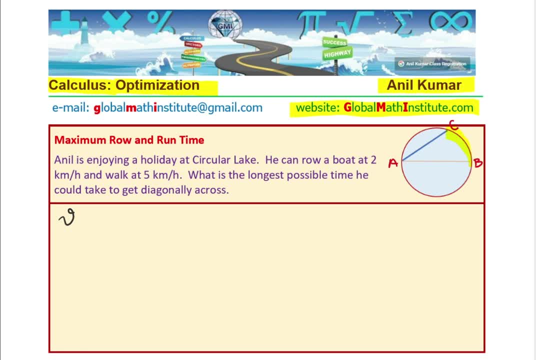 I could use walking W also. Okay. So let us say: velocity to row the boat is given to me, Okay, Okay. So velocity to row the boat is given to us as two kilometers per hour, And velocity for walking is given to us as five kilometers per hour. 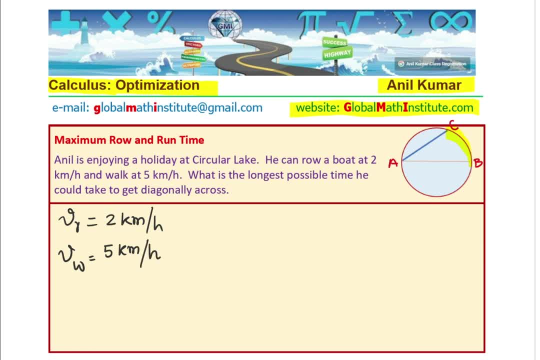 Right, And we need to. we are also given the radius of this circular lake, which is two kilometers. So this distance is two. The other one is also two. Let us say O is the center Perfect, Okay, Two kilometers. 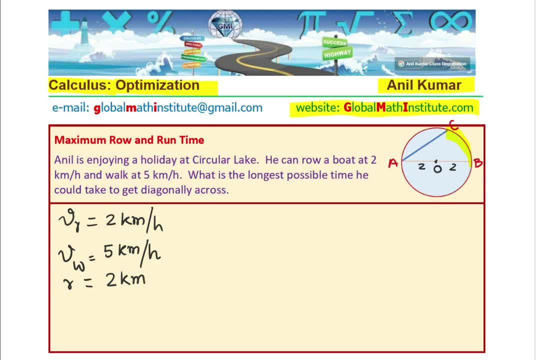 We are interested in time. Perfect. So two constraints are that he could go direct from A to B, boating or rowing, correct? So that will be one time And the other will be he could go along this circular path, semicircle, right. 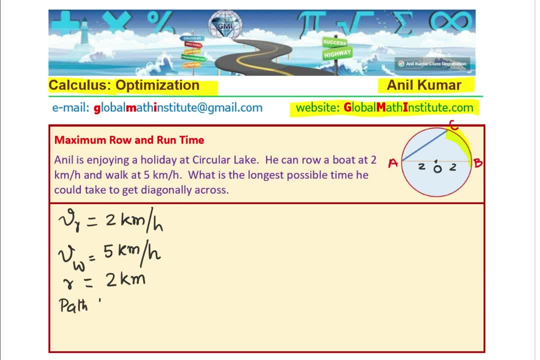 So I can say path one is rowing right Okay, A to B is distance of row from A to B right, And path two could be walking semicircle. So that is an arc ACB right Okay. 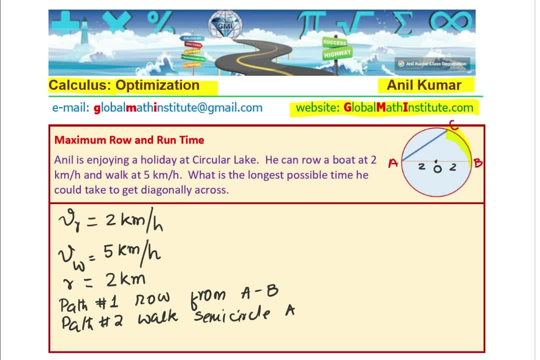 So we should normally write AB within arc, right, But it goes via C, right? Okay, That's fine. And third is that, as shown here, he could take ACB right. So path three is to row from A to C, right. 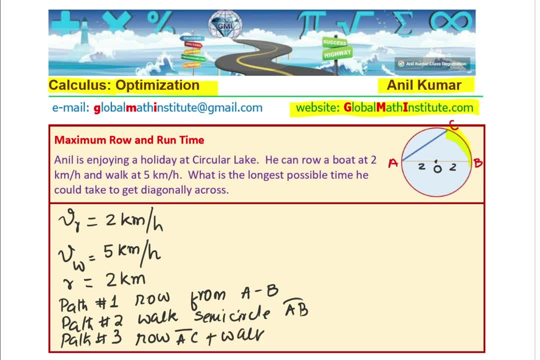 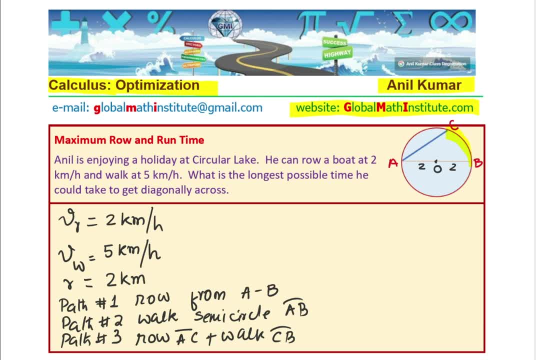 not difficult at all. we'll do that at the end, but first we need to figure out how do we get this part a, c and c b combination correct. that is what we need to figure out and that's the challenge. okay, so i hope you understand and appreciate this particular question. 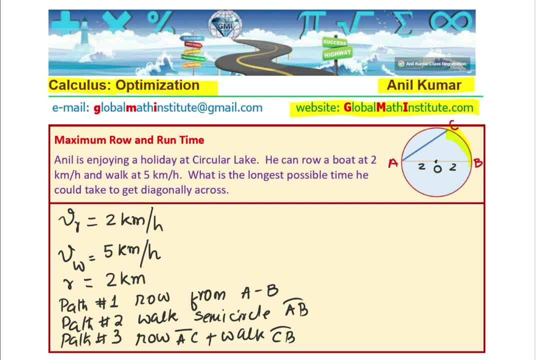 as much as i do and as much as my student who shared this question with me today. so what we can do is kind of do some construction here. join the center with c. now, if you remember trigonometric formula, we could do- um, we could use that concept. let us say: this angle here is theta. 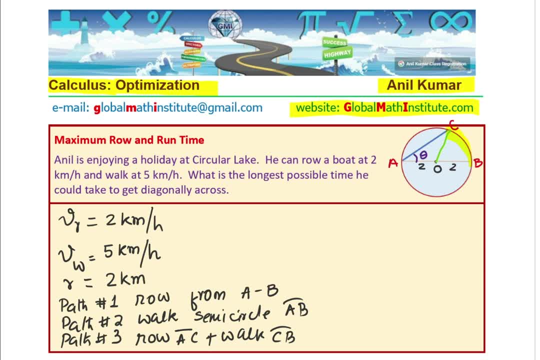 well, in that case the angle is in the center will be what the angle in the center will be: 2 theta. this is very important concept. this is one thing. So first concept which you need to understand is that angle at center is twice the angle on arc or circumference. this is one concept. 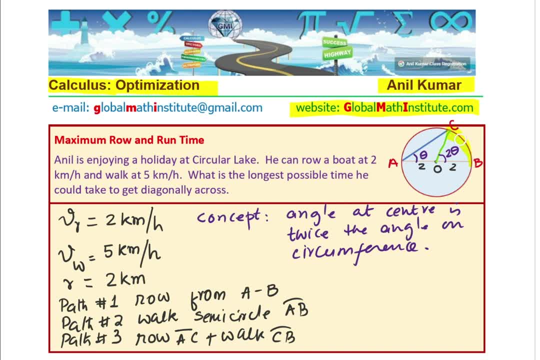 the second one is: how do we find arc length? So that is the formula. So arc length, let us say, if we have any angle given to us, you need to find the arc length. So it is important to review these things right before just getting. 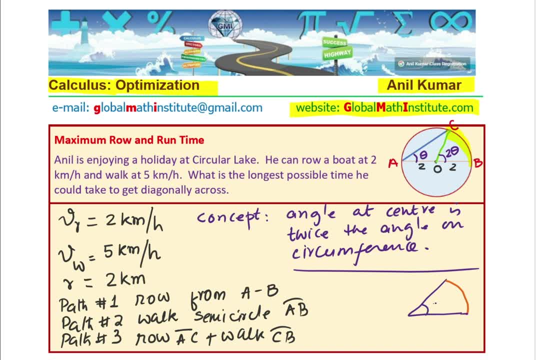 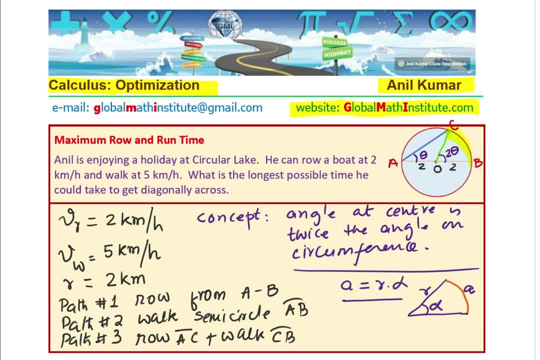 r times angle alpha. you see that. So that is the arc length and all measurements are in radians right. So note: the radius is the default unit. even in calculus, radians is the default unit. I see many books giving this angle theta in degrees right, in spite of the fact this is a calculus question. 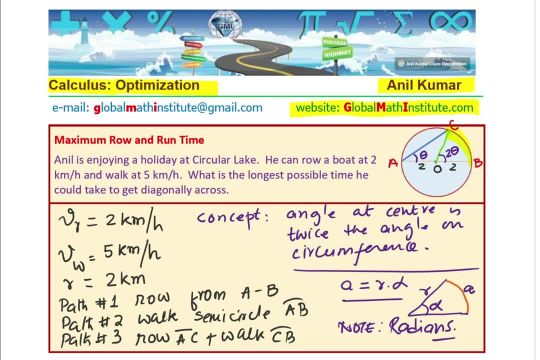 Perfect. So I think all the concepts required are right there on this particular screen, and so you are definitely in a position to find the solution. So let me give you this opportunity right. Well, in case you want to learn from me, you can always email me on this particular address. 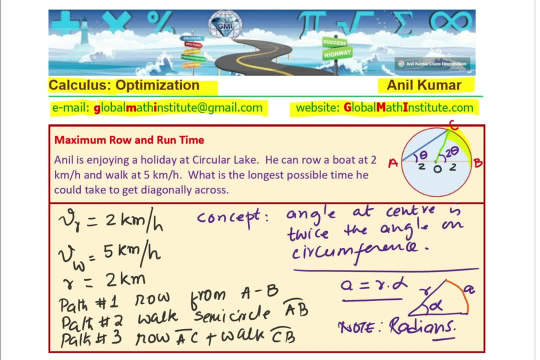 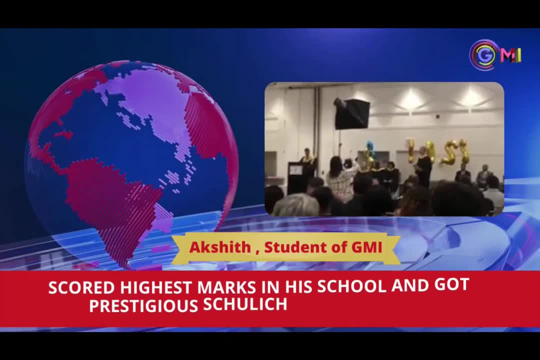 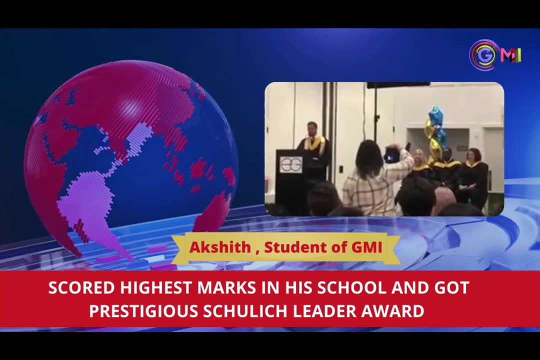 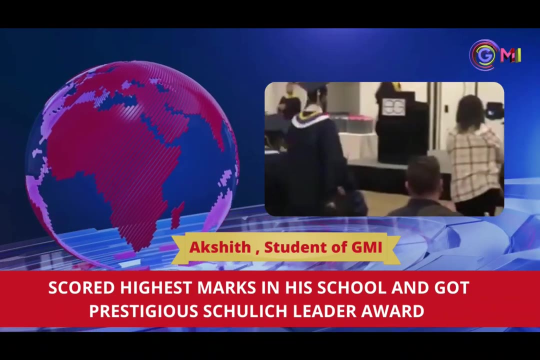 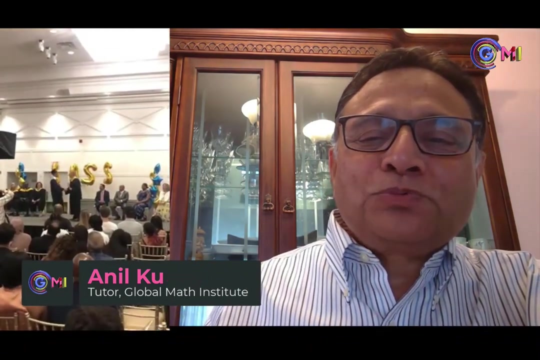 Most of my students are doing extremely well. some are right there on the top getting awards and scholarships- Perfect. The winner of this year's Certificate of Achievement Schulich Leader Award is Akshay Kandilani. Great, Our student, Akshay, gets highest marks and the most prestigious Schulich Leader Award. 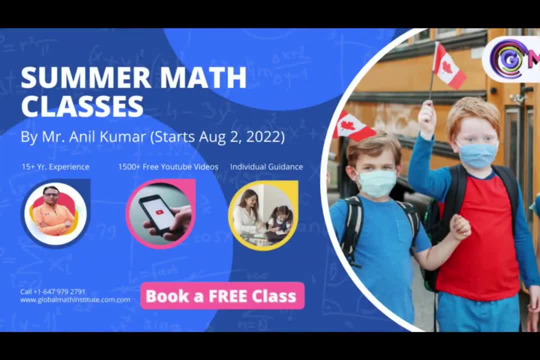 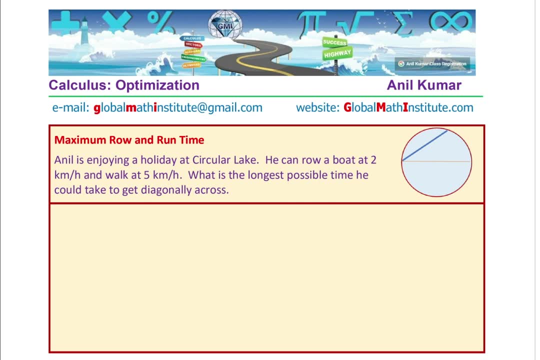 You can be there, Join our classes and excel. Let us now get all the relations. Here is our diagram. Let's fill in the information which we figured out. So Anil is on one end and he needs to go to B via C. 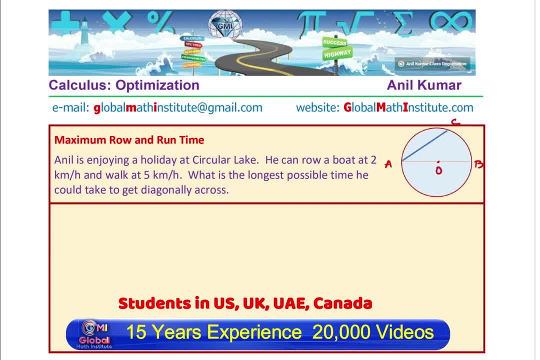 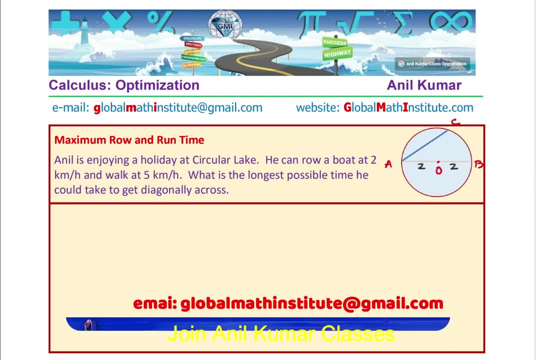 Center is given to us which is with radius of 2. So AO and OB is 2 kilometers. If I join O to C Then we get an angle right there at the center which is going to be twice the angle at the corner right on the circumference. 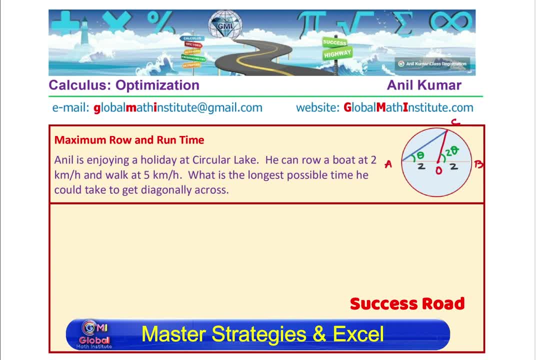 So that is the relation. We also know that OC should also be 2.. Perfect, Now, this is an isosceles triangle, correct? This is an isosceles triangle. So those two angles are theta and theta. 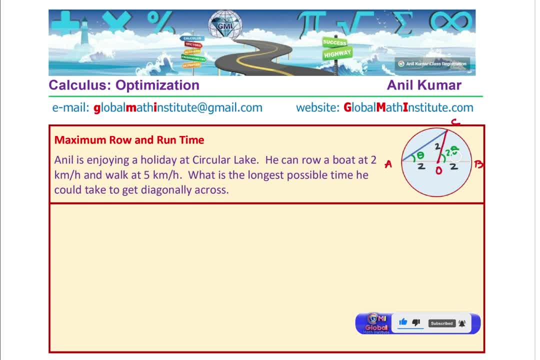 So the angle in the center will be 180 minus 2 theta, Even otherwise, you know, 2 theta is the other side. So this angle here, So we know that the angle AOC is actually equals to 180.. 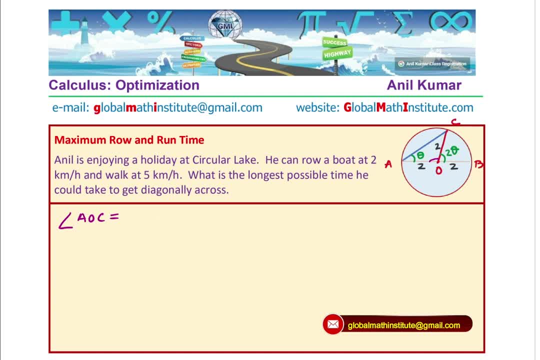 We are doing in radians, Remember that. So it has to be pi minus 2 theta, Perfect. So the idea is to find AC. So to find AC we can use sign law right, So we can write that AC over sign of the angle opposite, which is pi minus 2 theta is equal to CO. 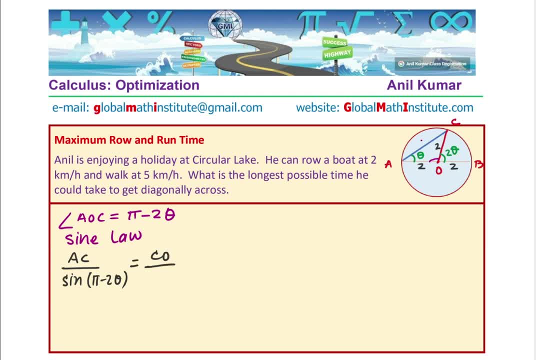 Over the angle opposite. is theta sign theta Correct, So AC is clearly equal to CO. is 2, right? So let me write 2 over sign theta, So AC will be 2 over sign theta times Sign. 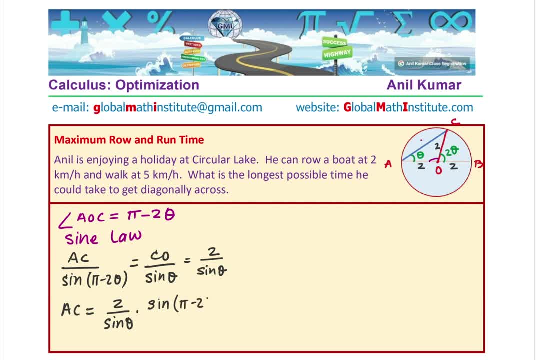 Pi minus 2 theta. So what is sign pi minus 2 theta? Sign pi minus 2 theta is sign 2 theta, Correct. So we get the value AC as equal to 2, sign 2 theta over. We have sign theta in the denominator. 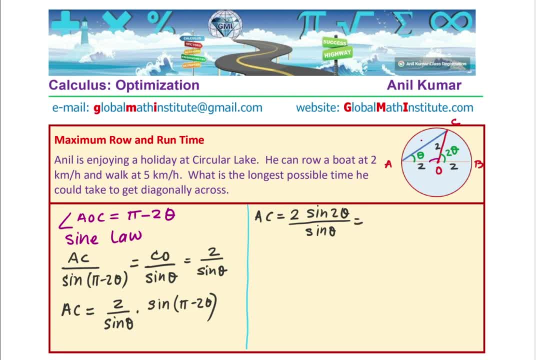 Do you remember the trigonometric relations double angle formula? Apply that. Okay, So it will be 2 times sign 2. theta is 2 sign theta cos theta, right? So it is 2 sign theta cos theta And we are dividing by sign theta. 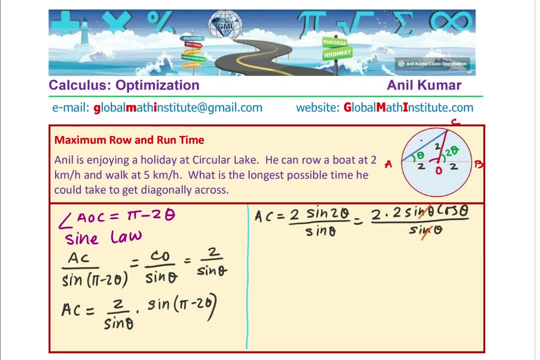 So we can simplify it by cancelling sign theta, which is common in both numerator and denominator. So we get the expression for AC As equals to 4 times cos theta. right, Correct. So that is how we get AC. We know how to find CB. 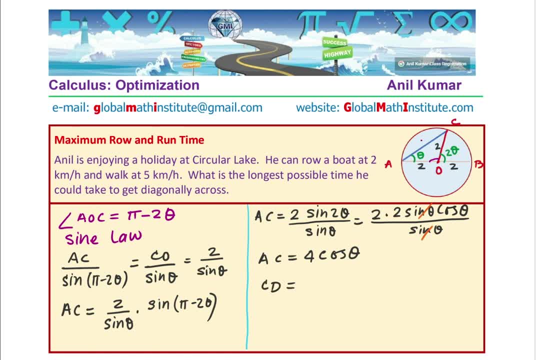 Can you tell me CB is arc length, arc theta, radius being 2.. So it is OC, Which is arc times, the angle between which is 2 theta, And this is 2 times 2 theta, or it is equal to 4 theta. 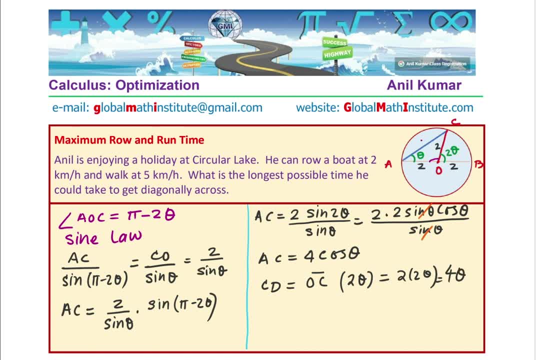 So we know both the lengths now, right. So AC, from sign law we just derived, is basically equal to 4 cos theta, And CB is basically CB C to B Arc length, Correct. So now, once we know that, the time taken is what, 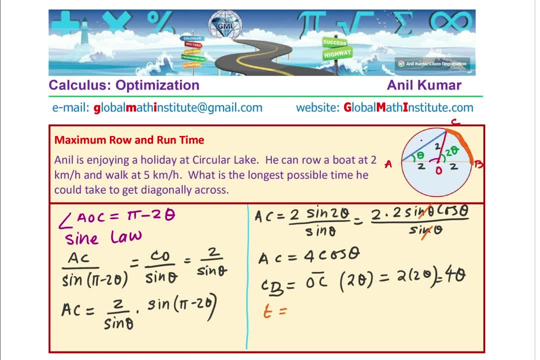 Time taken will be distance divided by speed. We know that the rowing speed is So distance, AC, which is rowing velocity of rowing, Plus CB. the arc with the walking speed, And that is, let us plug in, AC, is 4 cos. theta divided by rowing speed is given to us as 2 kilometers per hour plus walking speed of 5, right, 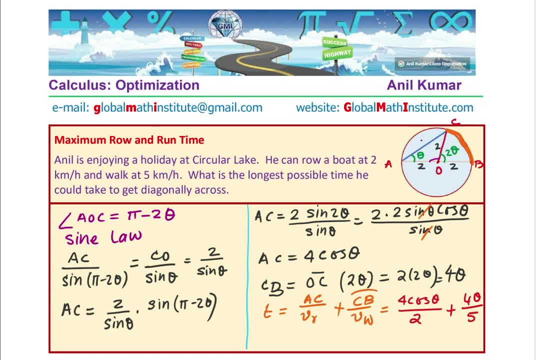 So it is 4 theta over 5.. So we now get an expression for time. Now it is very simple, right? You can find the derivative this and maximize the time Correct. So time is 4 cos theta over 2, plus 4 theta over 5.. 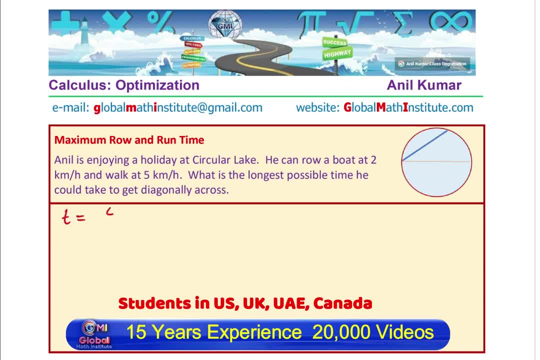 Let us go So: T time is 4 cos theta over 2.. And that is 4 theta over 5.. So let us differentiate time With respect to: With respect to theta, the angle, Since we are really interested in finding which angle, which path to take. 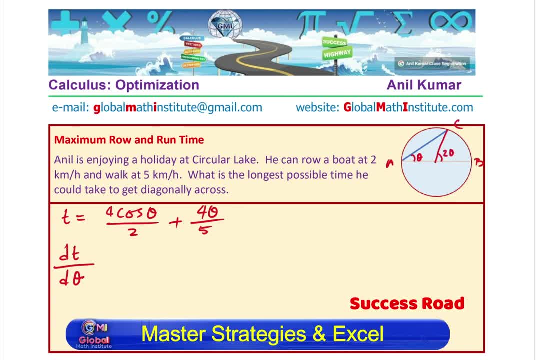 Correct From A to C and then to B, So that is like 4 by 2 is 2.. Right, So okay, Cos theta derivative is minus sin theta, So we get. Let me simplify it here itself. 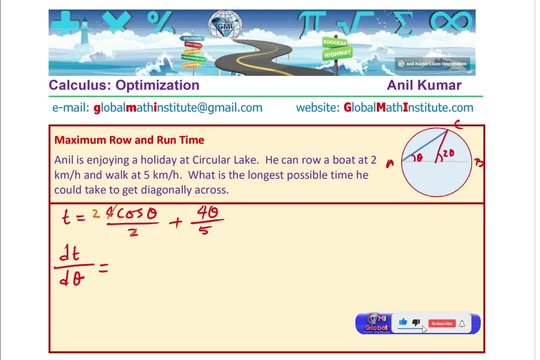 It will be easier, right? 2.. Okay, So we get 2.. And here the theta is 1., So we get 4 over 5.. So that is the expression. So really quick. 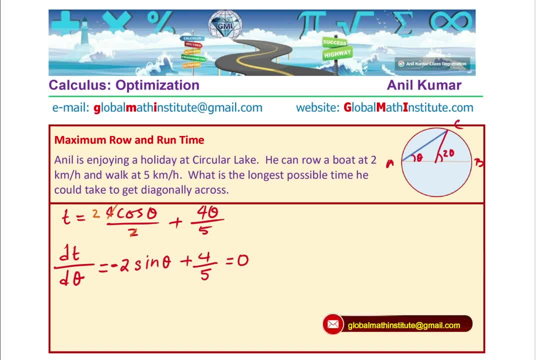 2. 0. To find the critical number right. So So that means minus 2 sin theta is or plus 4 by 5, I will write equals to 0, correct? Now we will solve for time. Is that clear to you? So we can write down 2 sin theta. 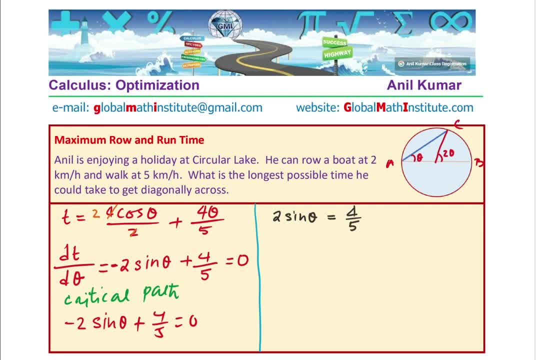 is equal to 4 over 5, or sin theta is equal to 4 over 5 times 2,, which is 4 over 10.. So theta will be sin inverse of 4 over 10,, which is 0.2, correct, So let us take calculator. 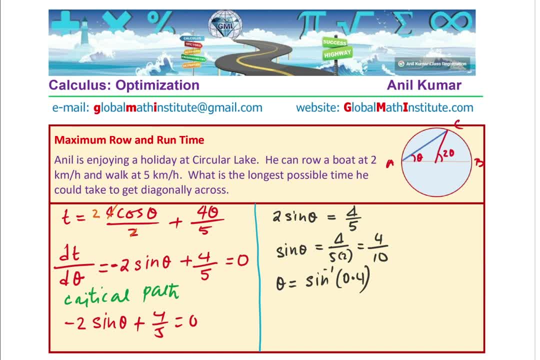 put it in radials first and then find the angle. So sin inverse 0.4 is equal to 0.41.. So 4, 1,, 1, 5, you can write Okay, So that. 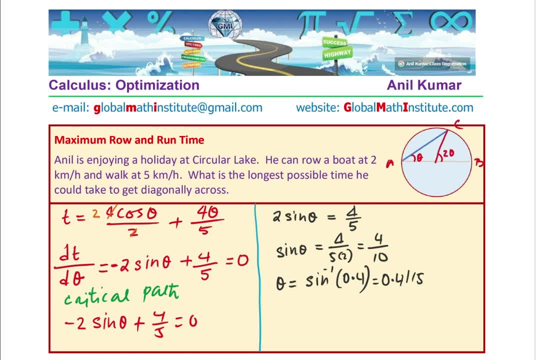 is what we get as the angle theta. Now we need to find what will be the time taken when that is the angle correct. So time t is given to you, So we can now calculate. So this is the time formula correct with angle of 0.4115.. So time will be time for the. 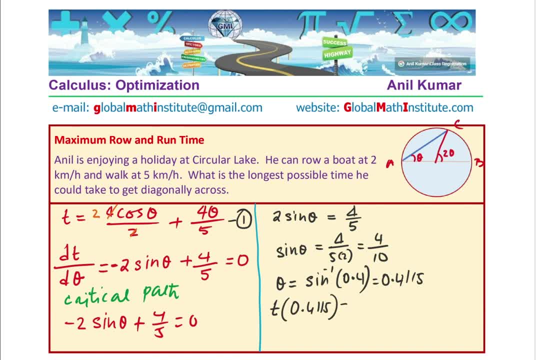 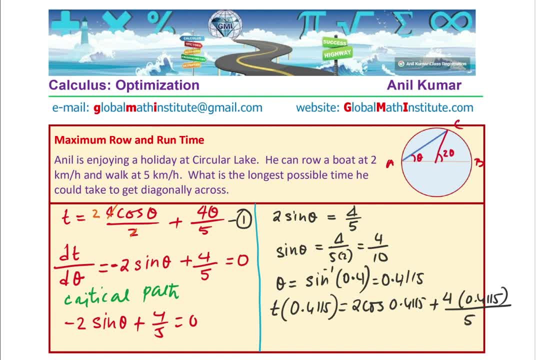 Okay, 5, plus 4 times 0.4115 over 5.. Let us calculate this stuff So, cos of the given angle, times 2, to this we are going to add: Thank you, Thank you, 4 times 0.4115 divided by 5.. 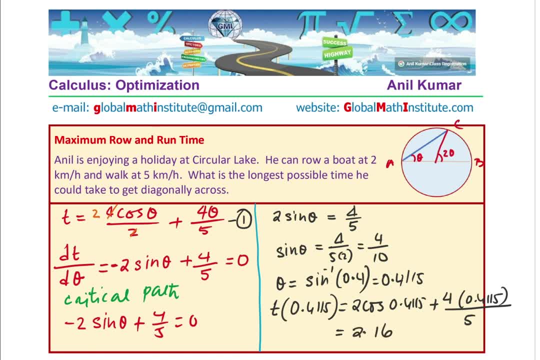 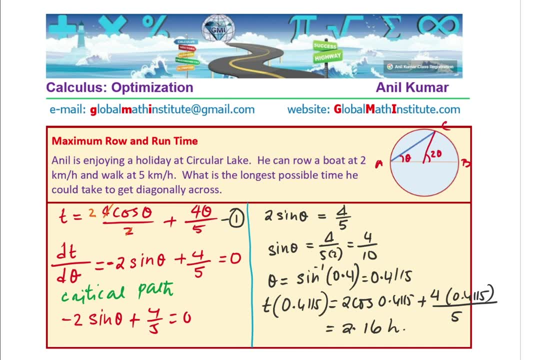 So that gives us 2.16 hours. So now we have found the critical time, which is 2.16 hours, when the angle here is 0.4115.. Let us now check whether this is the maximum time or not. Tell me how will you do that? 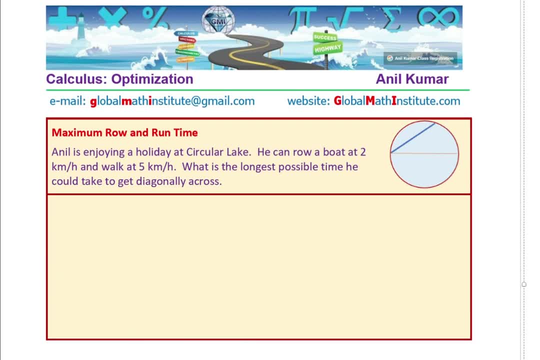 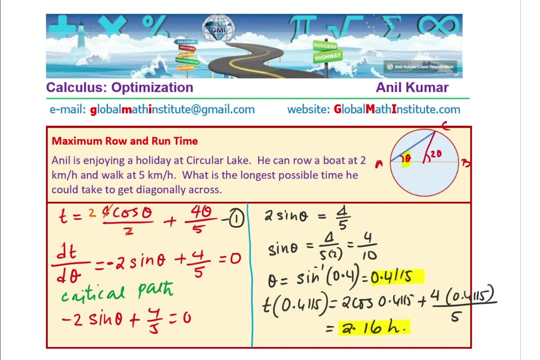 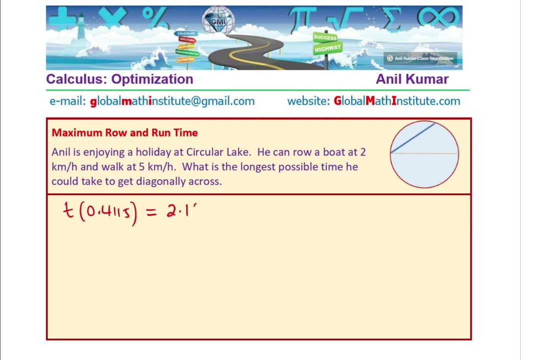 So well, we got the time for 2.16 hours, So now we have found the critical time, which is 2.16 hours, when the angle here is 0.4115.. In here this is 0.141, 152.16 hr. we should also convert this two hours and. 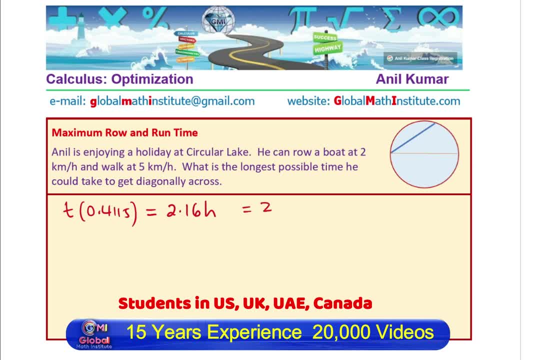 minutes. okay, So which is equals to 2 hr Plus 0.16 into 60 minutes, Do you understand? So that is easy conversion, Let's do it. so 0.16 into 60 will give you minutes, which is almost 9.6 minutes. so let's say: 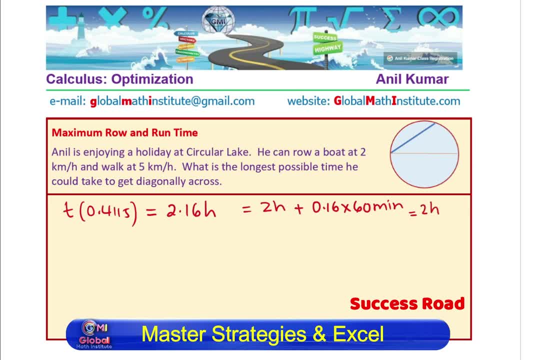 2 hours and let's say 10 minutes, correct. so that is the time which we have. now let us see what are the other times possible. so let's connect these dots: zero center a to b we want to go, and via c. so if i go direct, 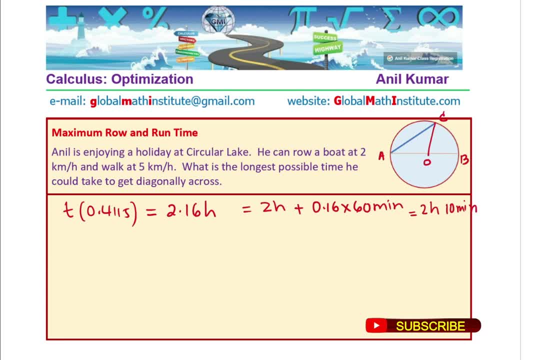 from time from a to b, direct right. a to b by rowing right. so if you want to row and go, then the distance is 2 plus 2, 4 right. so it is 4 kilometers divided by the speed of rowing, which is 2 kilometers per hour, and that gives you. 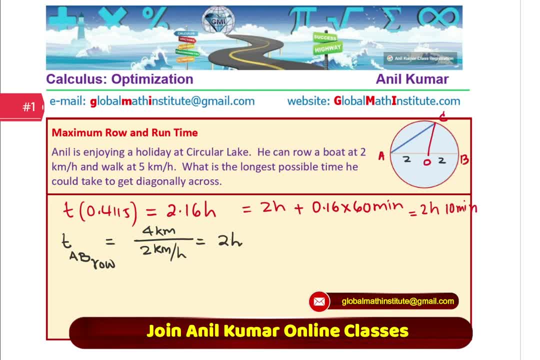 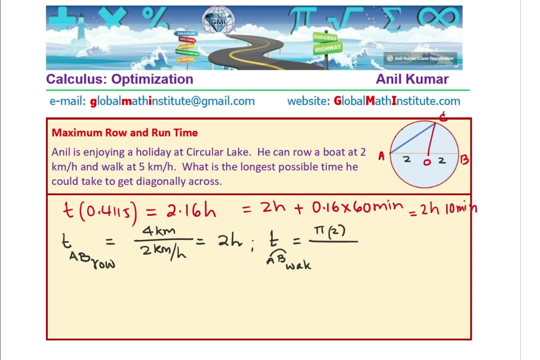 2 hours and if you want to calculate the time when you walk all the way right from that is the arc a to b, that is walking time- then this length is semicircle, right, so pi r r being 2 for you and the speed being 5 kilometers per hour. so let's calculate this walking time 5 kilometers. 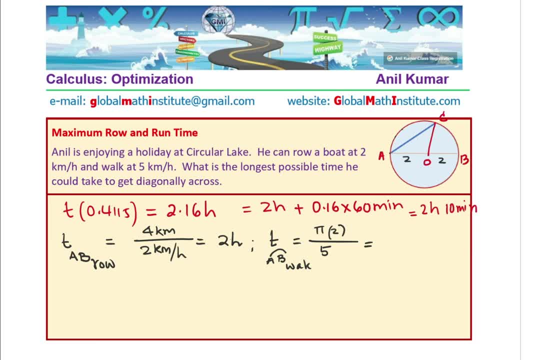 per hour. so it is 2 times 3.14 and we will divide this by 5, we get decimal value of 1.25, since walking speed is pretty high, so it is very less time in hours. we are looking for maximum time, correct. so maximum time indeed is 2 hours and 10 minutes, correct, and that is when Anil will row at. 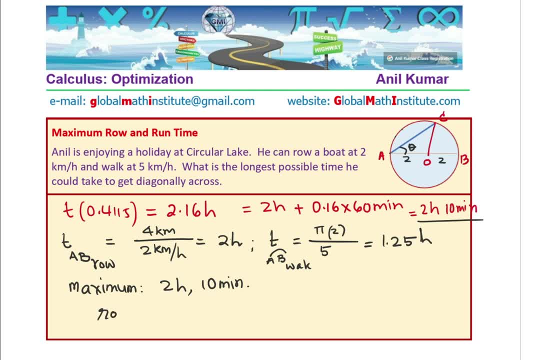 an angle theta, so that is to row at an angle of 0.4115 radius. you can also do this if you like. so introduction: no name, no interested, and I hope you enjoy this video there closely. so before we finish, please keep your questions in this type雅. 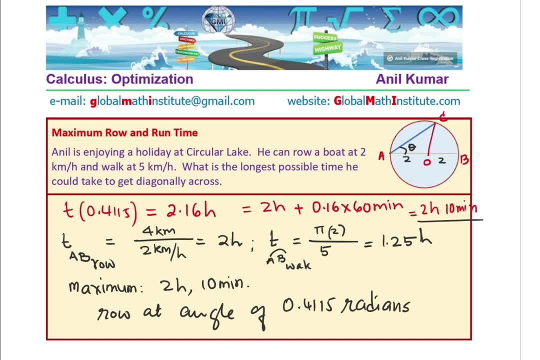 You can convert to degrees this radiance by multiplying by 180, dividing by pi right. So let's do that also: 0.4115 times 180 divided by pi right, And you get 23.57..